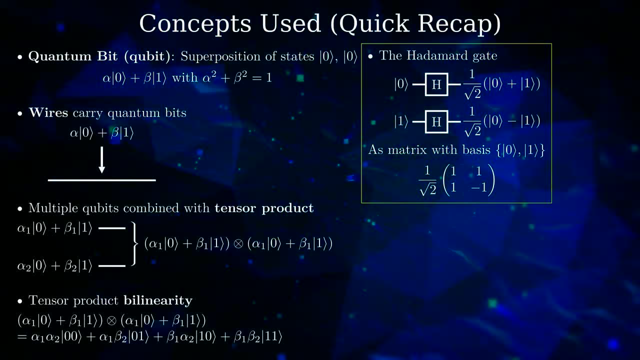 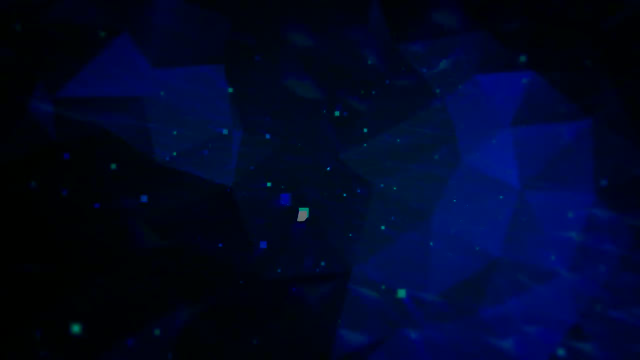 maps the states to certain superpositions. Places where we measure a qubit are indicated by a box containing a measuring device. In quantum computing, every operation and gate must be reversible and, to be more specific, must be a unitary operation. For that reason, a measurement is not considered to be a quantum gate. 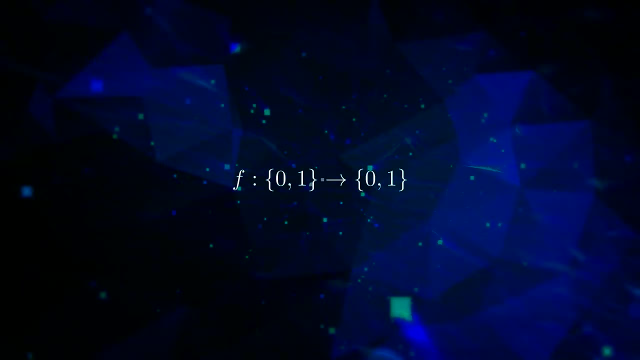 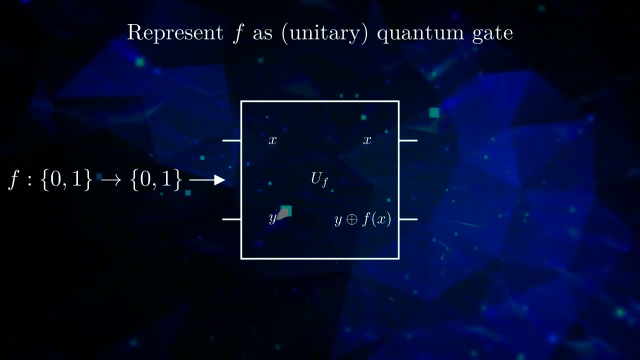 But coming back to f, A constant function is certainly not reversible. we do not know what the input was if we only know the result. We remedy this by wrapping a box around f that copies the input, But it actually does a little more. 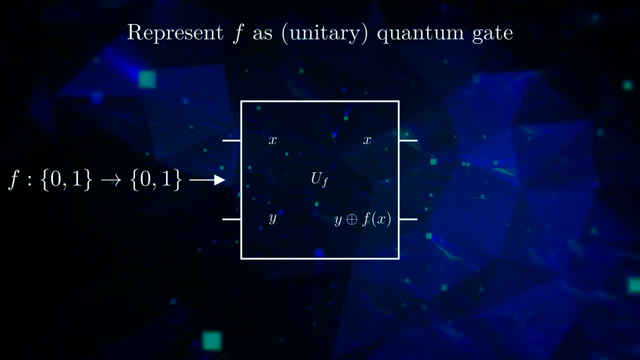 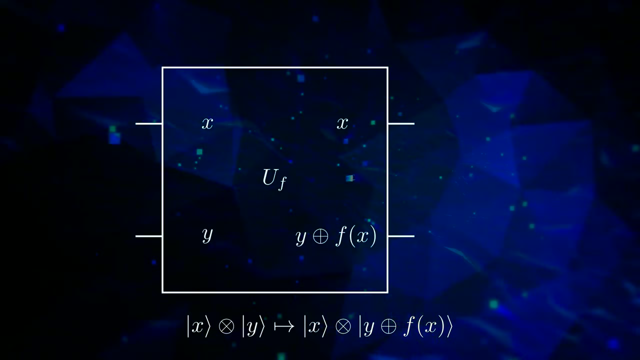 The output of f is combined with an input wire by adding their values modulo 2.. We write this as below with the tensor product. Now in the Deutsch-Jozsa algorithm, we use three Adama gates and we measure once. Let us go to the circuit. 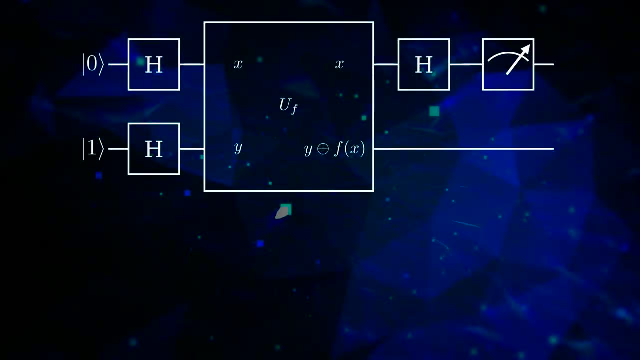 When we apply the zero and one state on the two inputs. First, the common state is described by the tensor product, Correct. After applying the Adama gates we get a new state that is the tensor product of two states that are superpositions of the basic states. 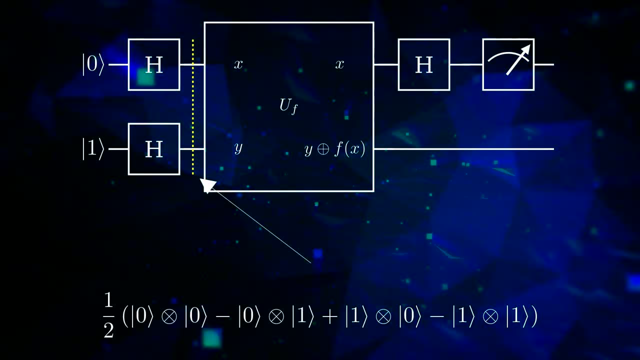 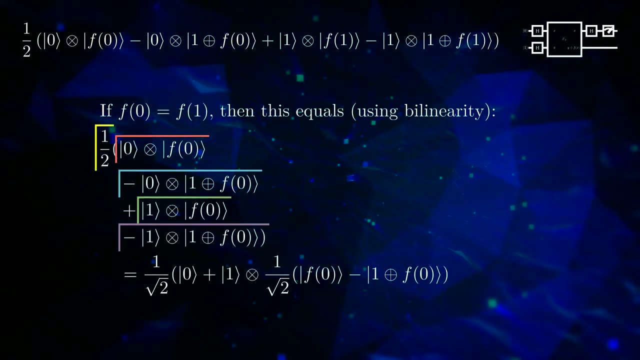 By using bilinearity this can be rewritten. Then we apply the quantum gate that encapsulates our function, f. Let us take a closer look what we get in either case, f being constant or not. Let us see: If f is constant, then by the loss of the tensor product we get the following: 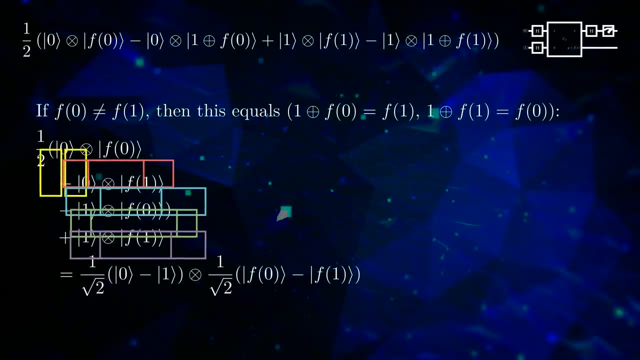 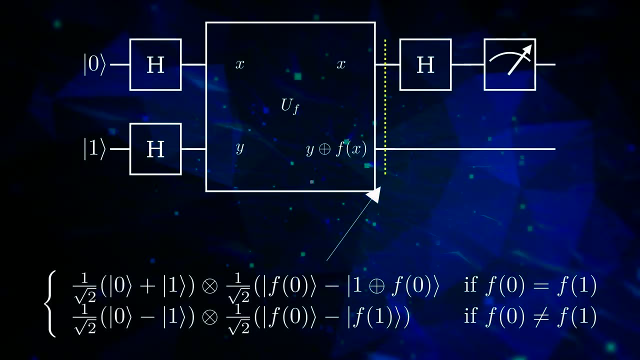 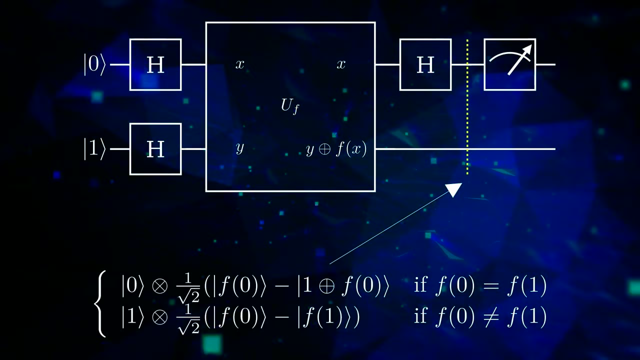 And if f is not constant, we get a different result. In total, we get the following state: After applying the Adama gates, we get a new state that is the tensor product of two states that are superpositions of the basic states. Let us see.